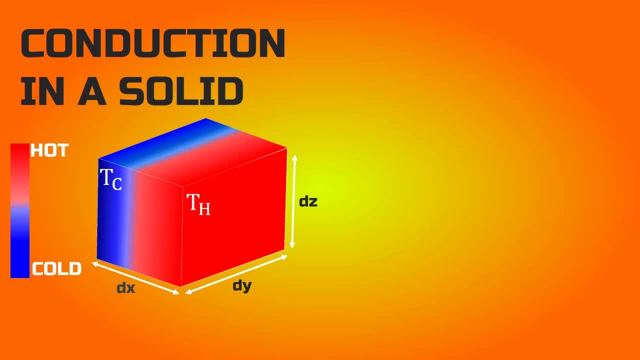 TH and TC are the temperatures of the hot and cold sides and Q is the heat applied to the hot side. Thermal conductivity is calculated from the Fourier's law of heat conduction, given by Joseph Fourier. Fourier's law states that the rate of heat transfer through a material is proportional. 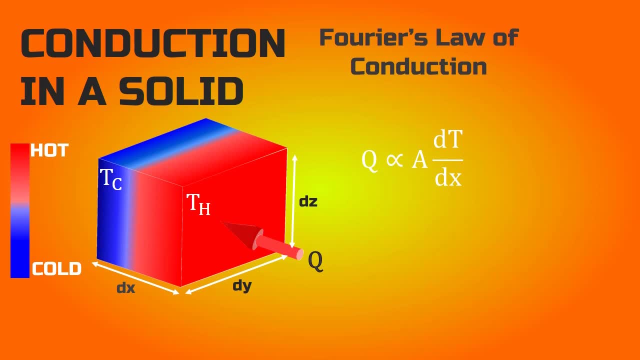 to the temperature gradient and the area normal to the direction of heat flow, where the proportionality constant k is the thermal conductivity. Now if we rearrange this equation, we get the formula for the thermal conductivity where A is given by the product of dy and dz, and dt is the temperature difference between hot. 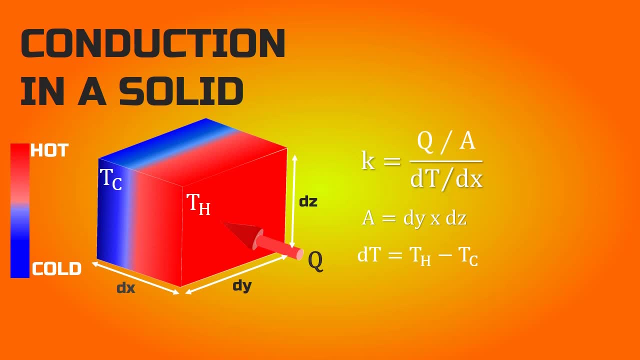 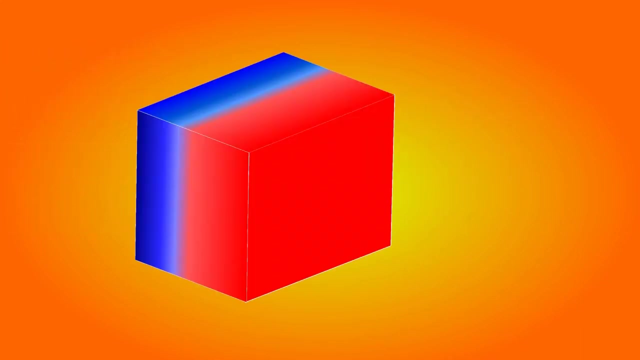 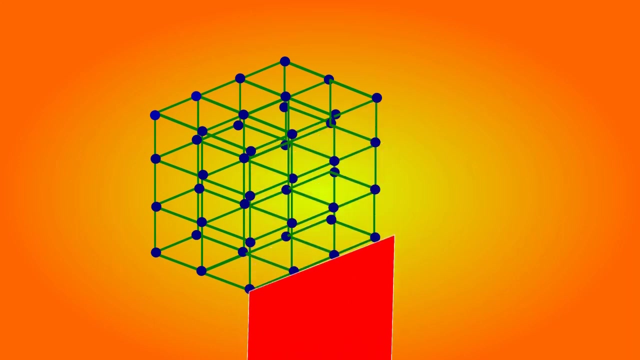 and cold sides. Thermal conductivity has a unit of watt per meter kelvin. Now we will see what drives conduction in solids. Here we see a hot cuboid. if we cut it open, inside we will see a solid skeleton which is known as lattice structure or atomic arrangement of a material. 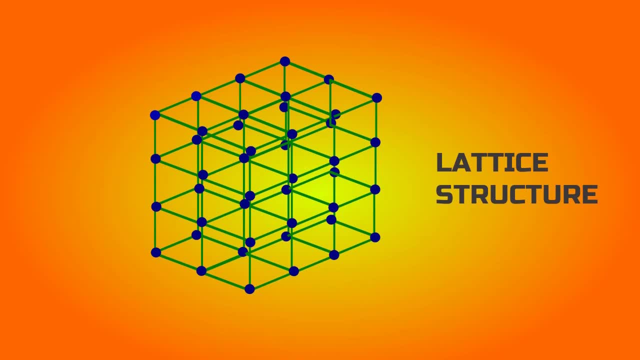 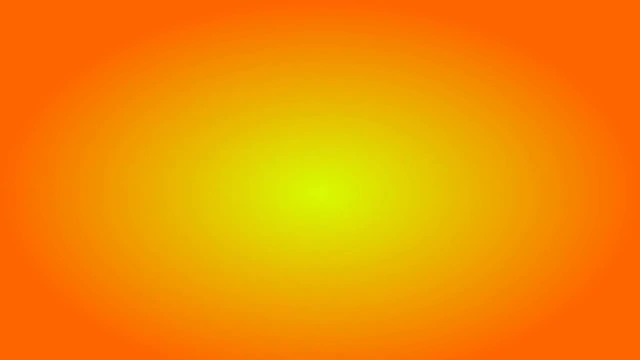 This is one of the things which will drive conduction in solids. Next is the migration of free electrons, which can also cause conduction in solids. Now let's see what happens if we cut a hot cuboid. Next is the migration of free electrons, which can also cause conduction in solids. 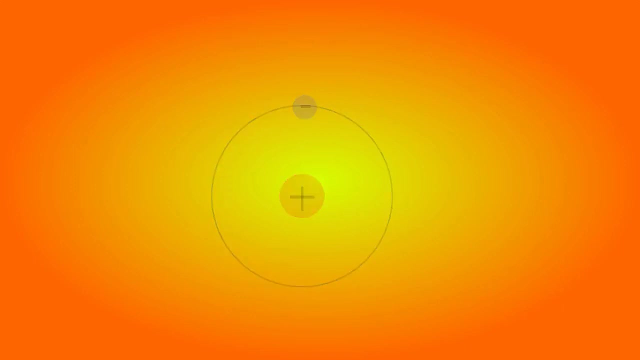 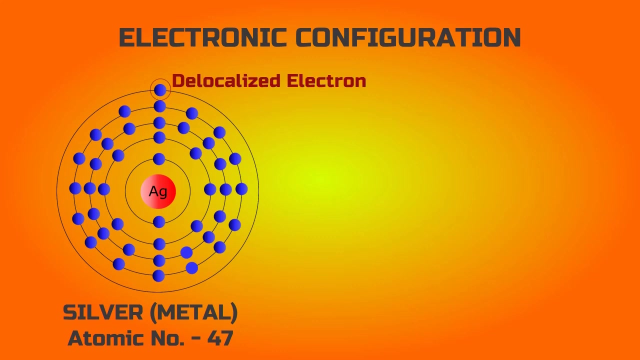 can also cause conduction in solids. Let's see at the electronic configuration of a metal, silver. You can see that its outermost shell has one electron. This is known as delocalized electron. Silver atom can lose this electron to become stable, and these are the free electrons which can then transfer heat inside the. 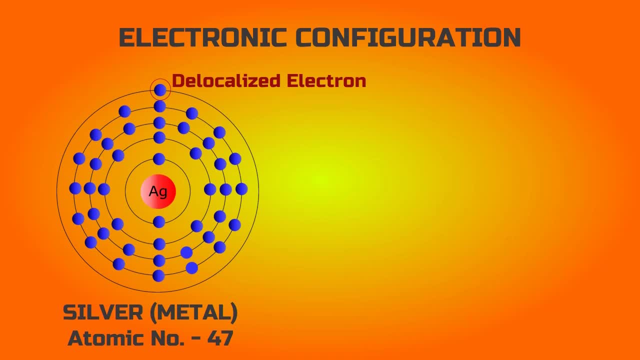 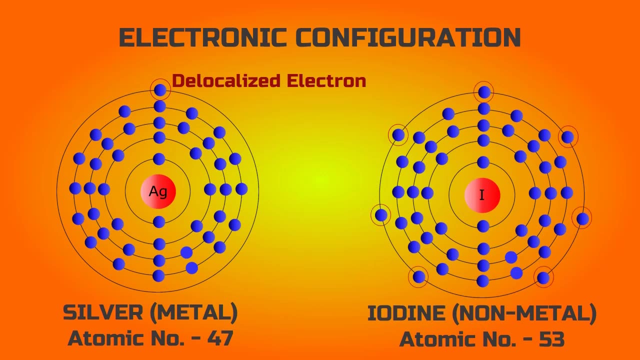 metal. Opposite to that, a non-metal such as iodine has seven electrons in its outermost shell and will not easily lose electrons to become stable. So non-metals do not have free electrons for conduction. Now we will see how conduction takes place in metals. 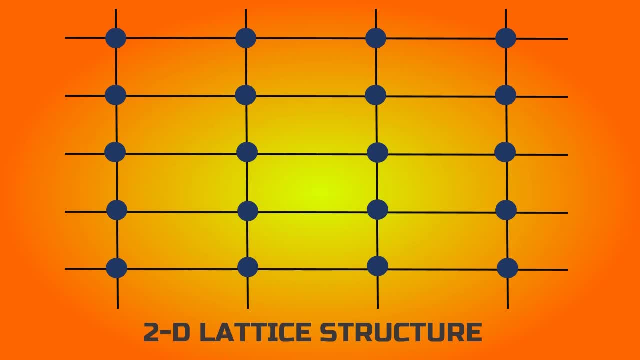 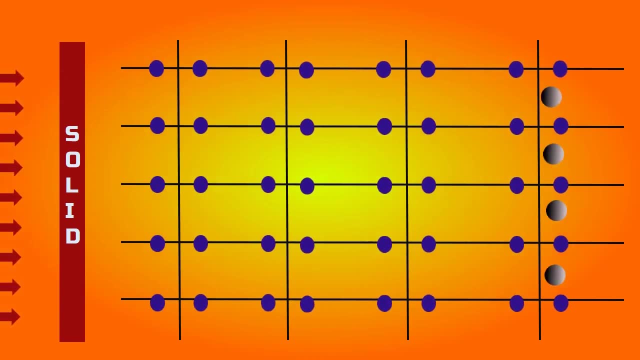 What you see here is a 2d lattice structure of a material. In metals, conduction takes place by lattice vibration and electrons. When heat is supplied to a metal, its lattice structure starts to vibrate about its original position and transfers the heat energy. This is known as lattice. 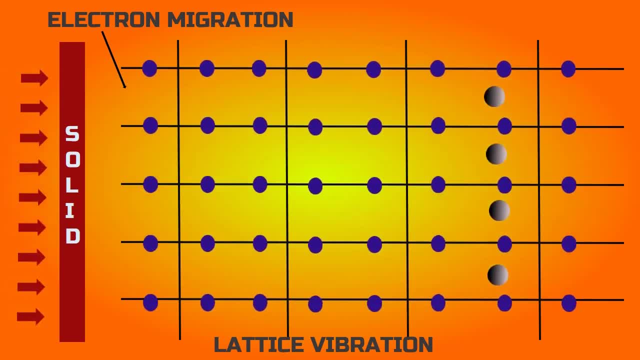 vibration, which is shown here in blue color. Also, since metals have lots of delocalized electrons, shown in black color, they also strike through non-metals, migrate and transfer the heat energy. in pure metals, electron contribution is the most dominant. now that we know how conduction takes place, let's look at 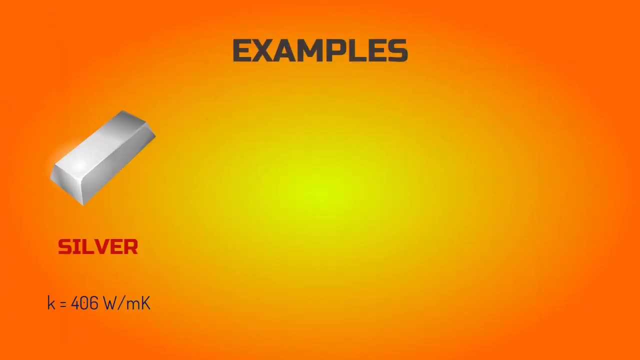 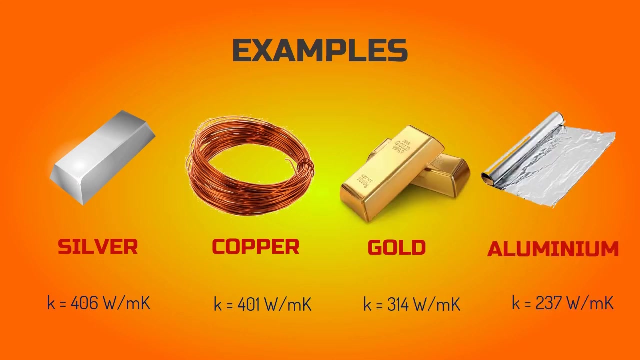 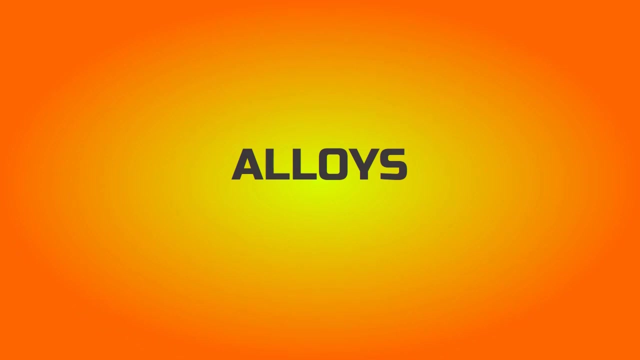 thermal conductivity values of some metals. now let's move to alloys. alloys, as we know, our combination of two metals. so what should happen if we produce an alloy by combining two metals of higher thermal conductivity values? let's take aluminium and copper and we get a resulting alloy, bronze, which tends to offer a 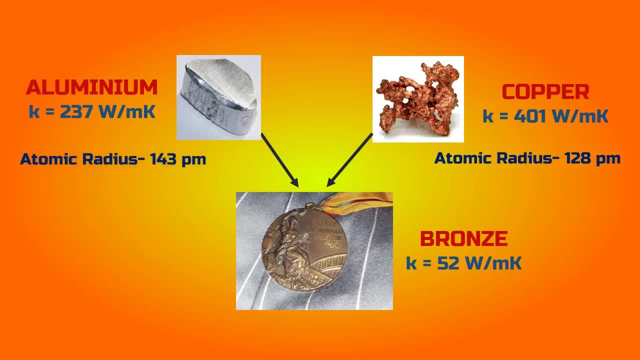 range of high thermal conductivity values and we get a resulting alloy, bronze, which tends to offer a lower thermal conductivity value than the pure metals itself. it's because atoms of different size will vibrate at a different rate which changes the pattern of thermal conductivity. this results in less energy transfer between. 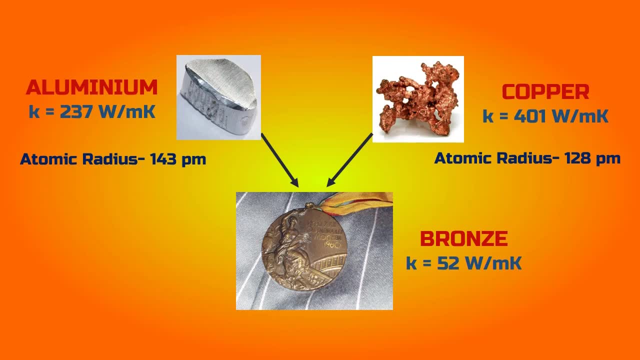 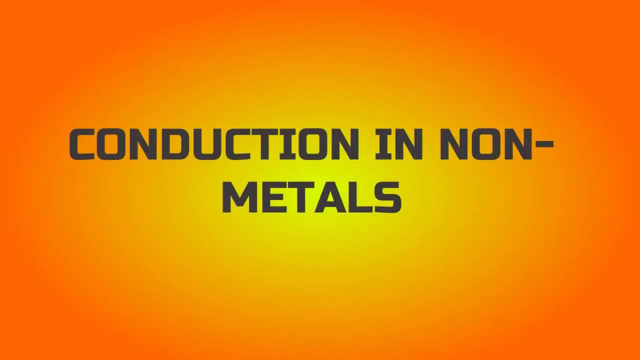 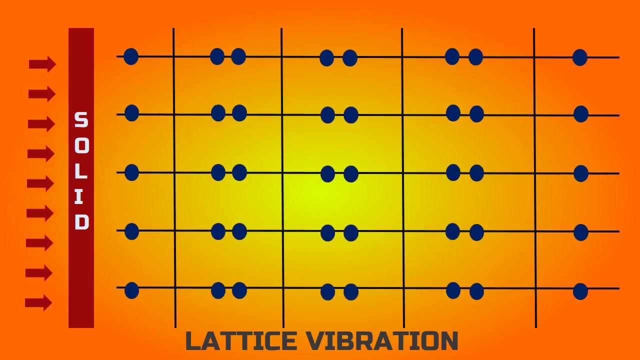 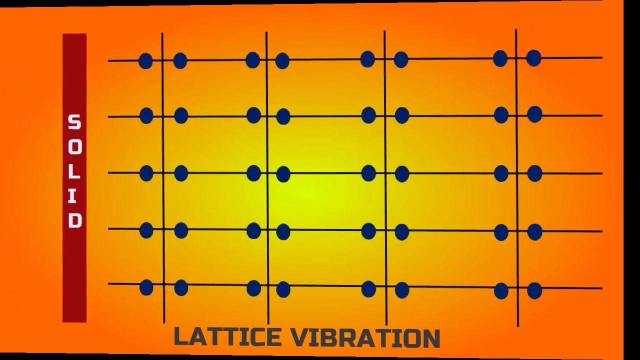 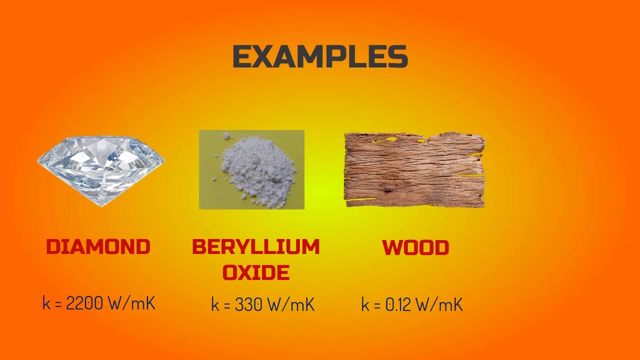 atoms and therefore there is less thermal conductivity. now let's move to nonmetals. as we have seen earlier, nonmetals do not have any free electrons for heat transfer, so conduction in nonmetals is generally dominated by lattice vibration. now let's look at some examples of nonmetals. you can see here that diamond has a very 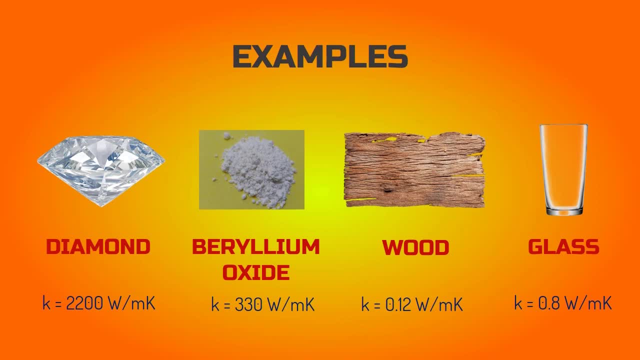 high thermal conductivity value, exceeding that of silver. this is due to its very highly ordered lattice structure rather than an amorphous material like glass. this also demonstrates the effect of arrangement of lattice structure on the thermal conductivity of a metal material. lets see an example of a SQL crystal pattern. 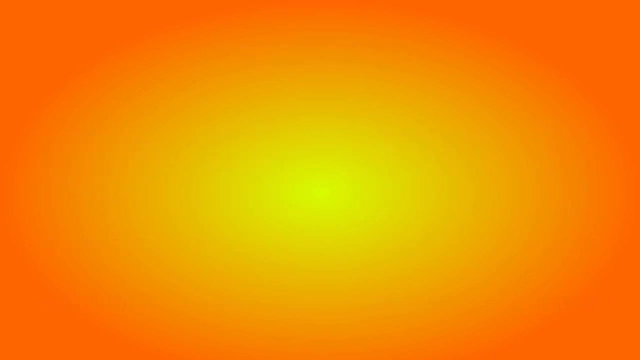 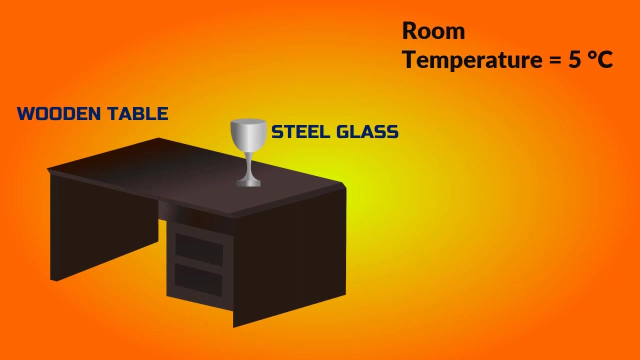 is calculated for a happening state of high temperature and pressure test. now let's take a situation from your day-to-day life: a wooden table in the room having a steel glass over it. if its cold outside, say it's at five degrees Celsius, we can assume that the steel glass and the wooden table are both at